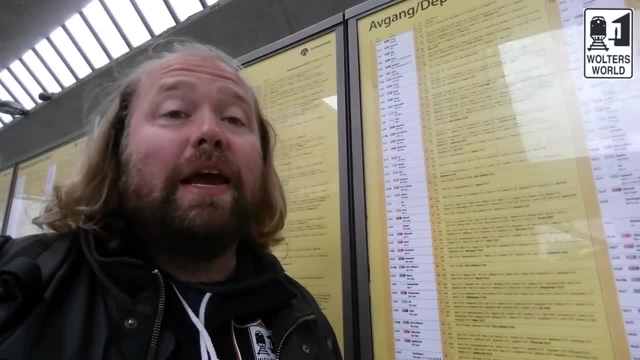 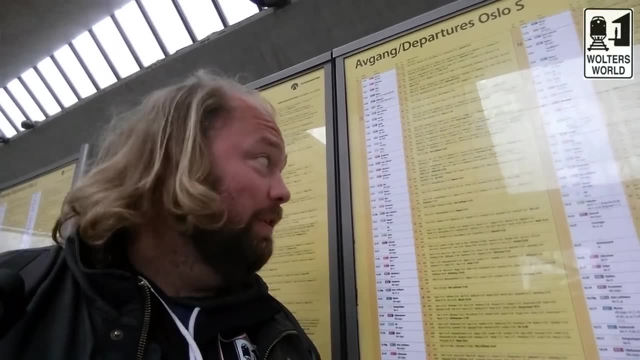 out our website at waltersworldcom. we're also on Twitter and Facebook and we really appreciate licensed subscriptions. we've got all kinds of these short little tips and longer tips as well for traveling. and bye from Austria, I'm going slow and I'm getting ready to take my train to Lidlstrum. Bye.